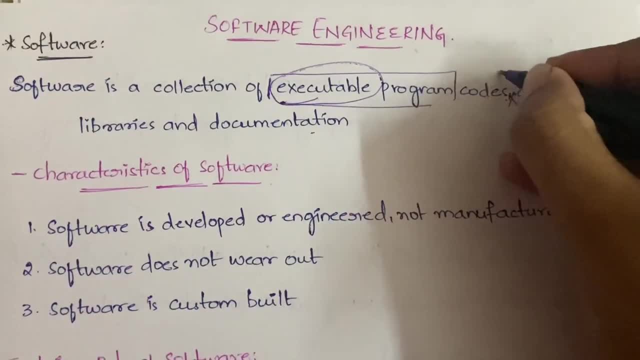 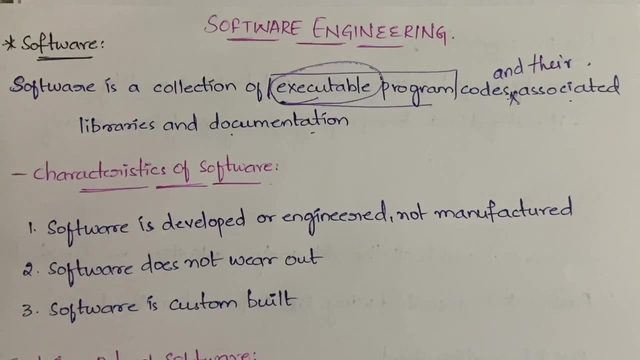 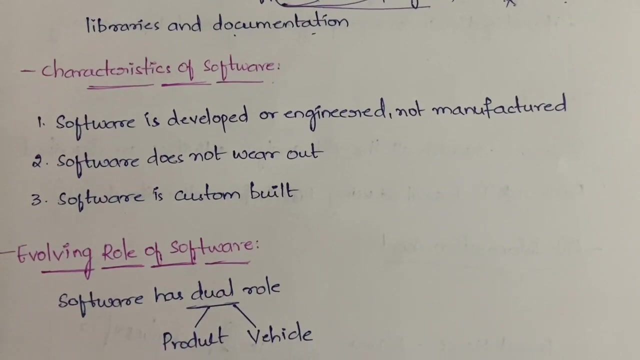 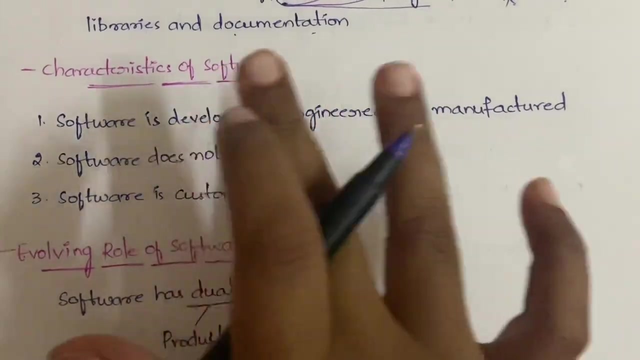 the libraries, program codes and their associated libraries and documentation. So all those things will come under the software itself. Got it Now. so what is the characteristics of- sorry, what are the characteristics of software? Let us see now. First: software is developed or engineered, does not manufacture. So what do you mean by development? and what do you mean by manufacturing? Right, First, development is nothing but. 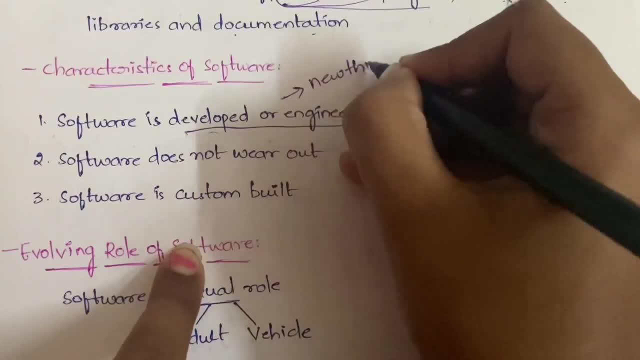 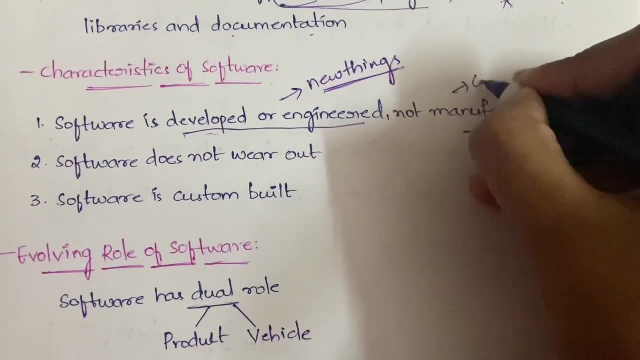 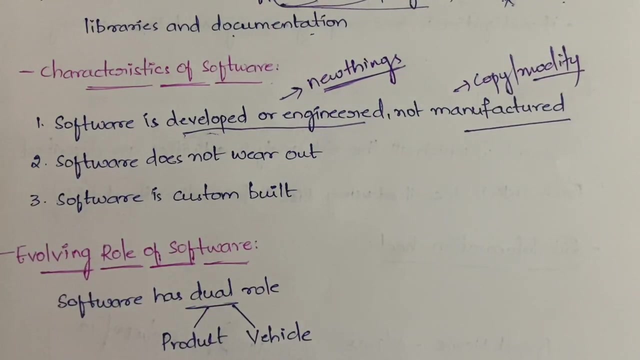 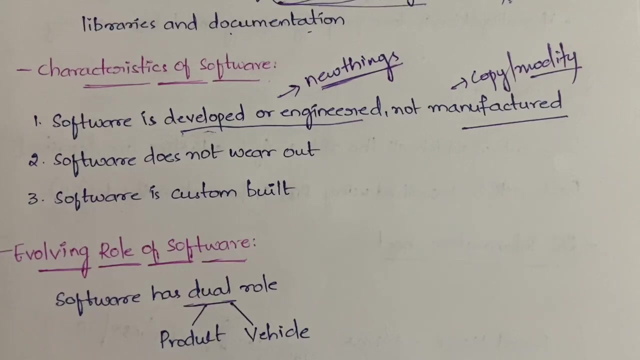 completely new things. you will create Entirely new things. you will be creating and developing or engineering. But in case of manufacturing, you will not do that. You will be copying the existing one or you will be modifying. that is, you will have a prototype, you will have a design, you will have a model, blueprint kind of thing, And you will be following it in manufacturing. But in case of engineering or development, you don't do that. you create all new things. Okay, so that is the difference between development and manufacturing. Got it? And 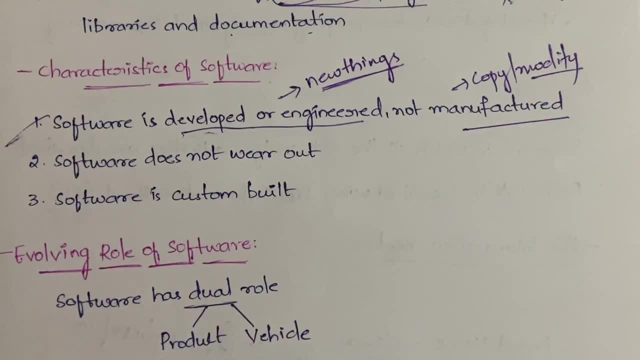 next software does not wear out. wearing out is nothing, but See, on time you cannot use it. Suppose you purchase new clothes, Then after, if it is branded, then maybe you can use it for one or two years, then later on you cannot use it Right, Even shoes also, or you know any footwear, kind of. so you cannot use things. as time passes. some things, not all the things, So in case, 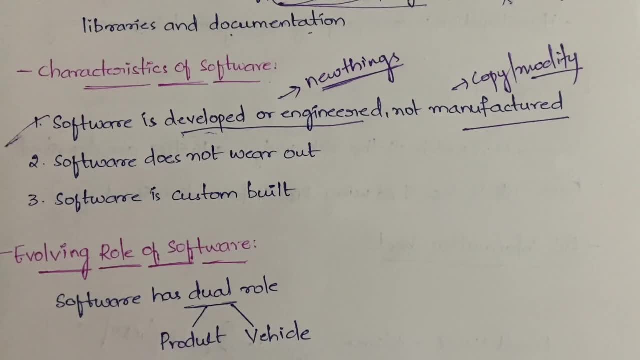 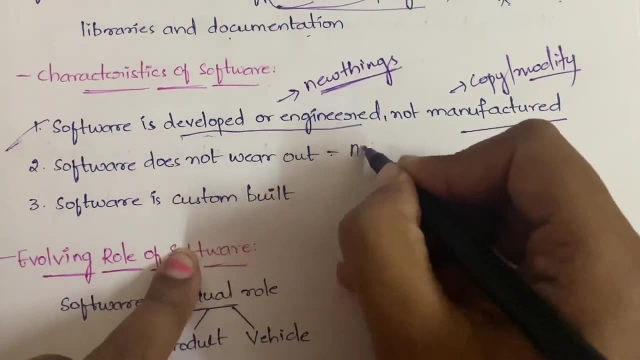 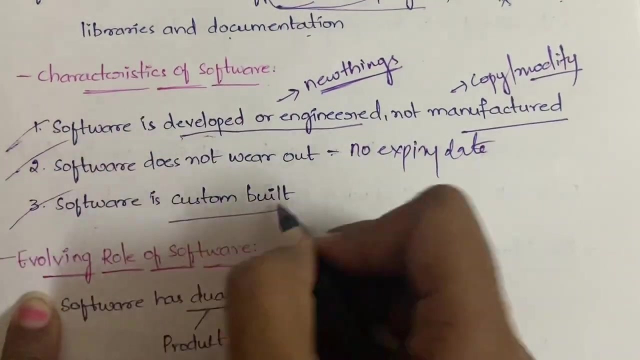 of software. it does not vary out, which means you can use it, uh, forever. there is no expiry date for this. yeah, this is very no expiry date for a software. okay, next, software is custom built. custom built is nothing but, um, you can say also customer built, that is, according to the choices of the customer you will be doing. 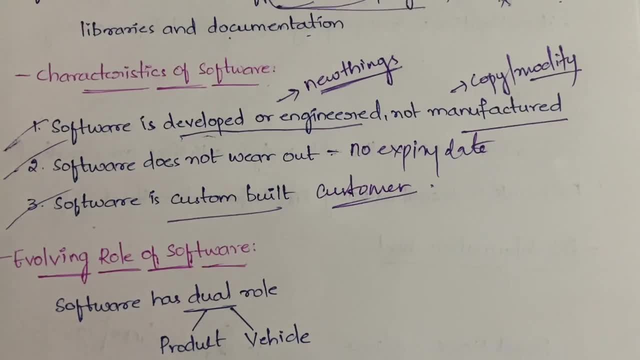 it see, suppose, suppose. let us take any example of some food items or anything. they are already manufactured. you go to the supermarket, you pick them and you'll use it right. but software is not like that. customer will ask that i want so and so, uh, i have. so you know the customer will give. 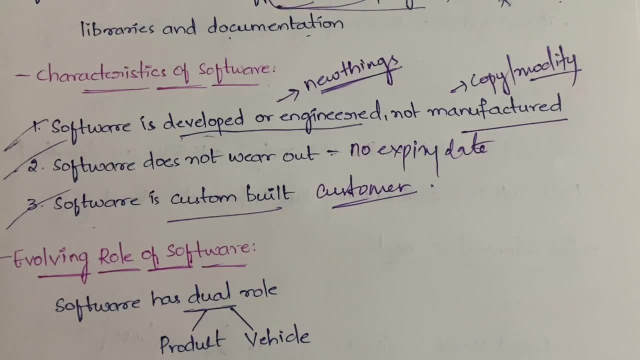 all their requirements, all their specifications, according to the choices of the customer. software is being built right, not according to first. initially, a software is built and the customer has to come and purchase it. it is not like that. so in most of the cases the software is custom. 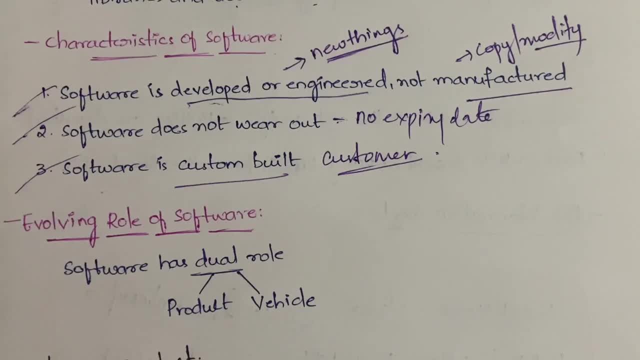 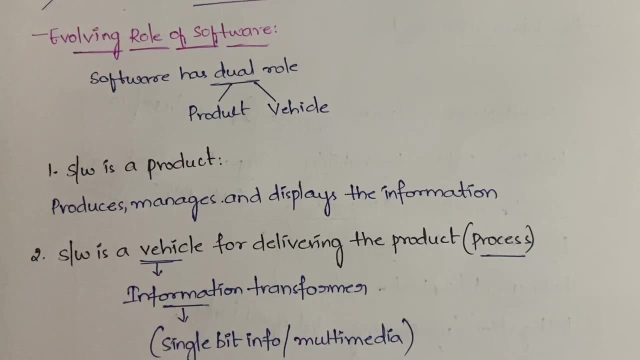 built only, that is, according to the choices of the customer. we will be building it, okay. next, evolving role of the software. so evolving role of the software is nothing. but a software has exactly two rules: one is the product and the other is the process. okay, and see dual role it. 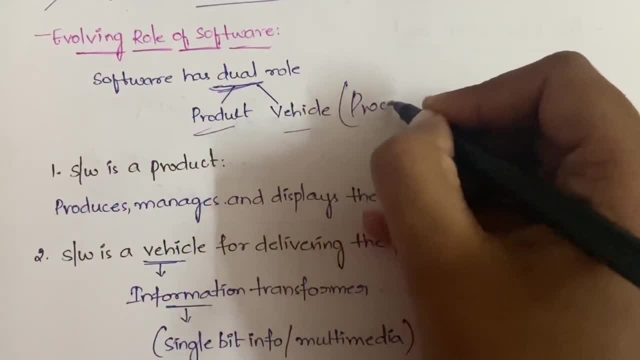 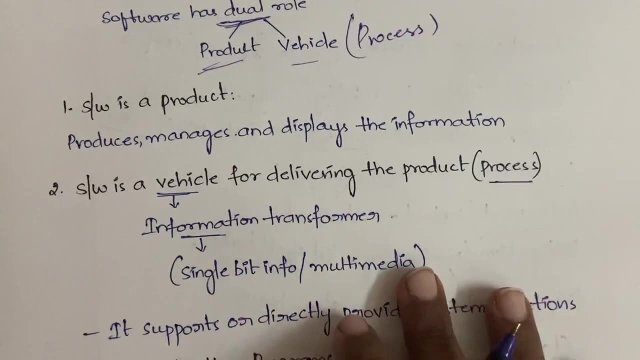 has two roles: product and vehicle. vehicle is nothing but the process, that is, vehicle for delivering the product. okay, so first of all, uh, software is a product. how do you see software as a product? i'll tell you: it produces, manages and displays the information. right. so as a product. 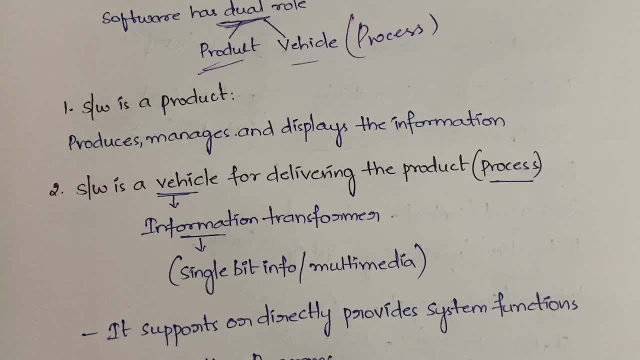 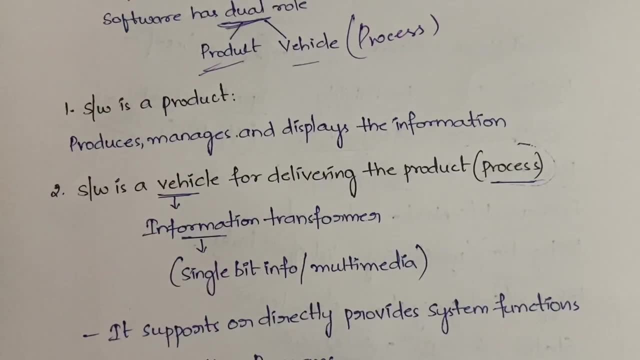 the software will be producing and managing and displaying the information. and software is also a vehicle for developing the product, which is nothing but the process that is, you have manufactured a product and you have to. uh, if you just keep, keep it in your industry or keep it in your factory, sales will happen. no right, you need to sell it, you need to make it advertise to. 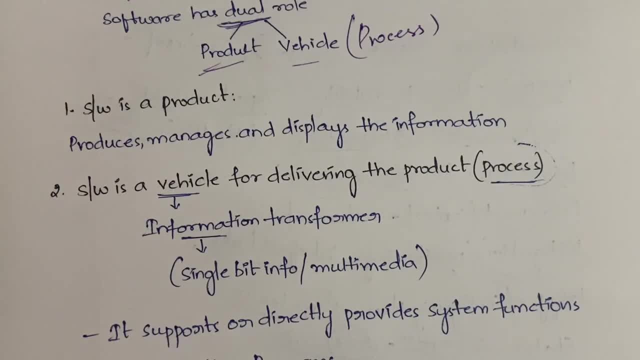 the customers. so for that, what you need, you need to deliver, you need to book a transportation. you have to go to the retailers or the wholesalers, you have to do it. you have to go to the distributors, you have to go to the advertisers, you need to do it. 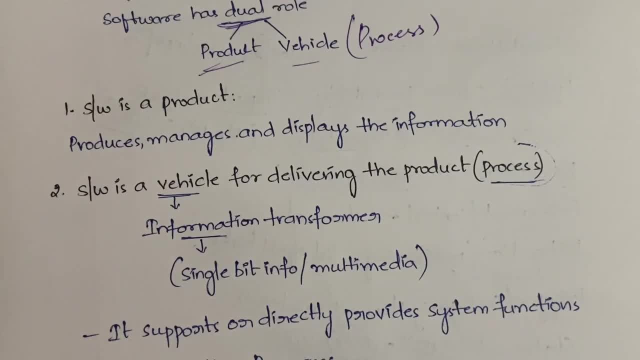 be doing a lot of work right. so the same way, if you just prepare a software and sit, it will not work. you need to deliver the software to the customer right and you have to take the review from the customer. so it was all about a process. so it is a vehicle or for delivering the product. 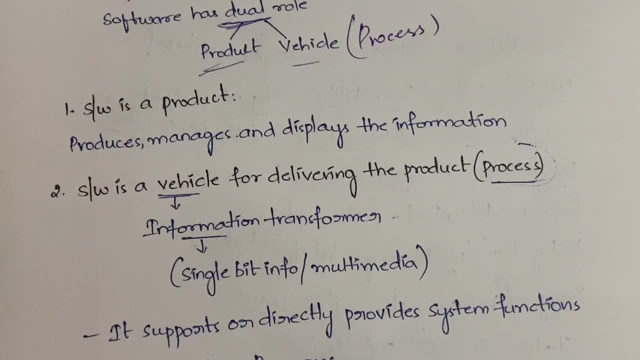 both, both roles. software only will do, and at a point it will act as a product, at a point it will act as a process, according to the situation got it vehicle is nothing but the information transformer. right, it could be anything. the information could be a single bit information, or it can.